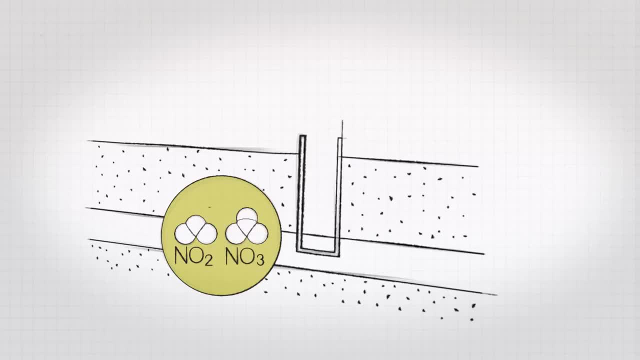 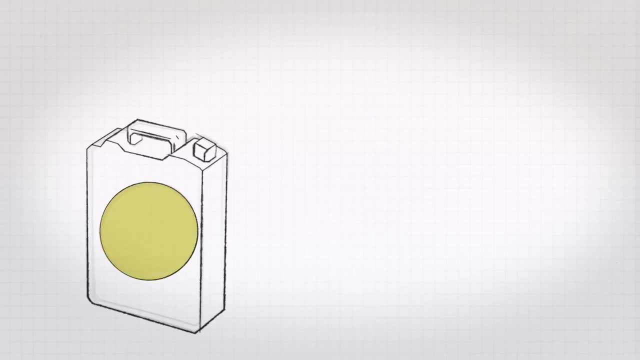 to nitrite and nitrate. High concentrations of both compounds are harmful to humans. Urine can also pollute the air. When urine is not properly handled and stored, it releases ammonia into the atmosphere. The degassing of ammonia can have multiple negative effects on human health and the environment. 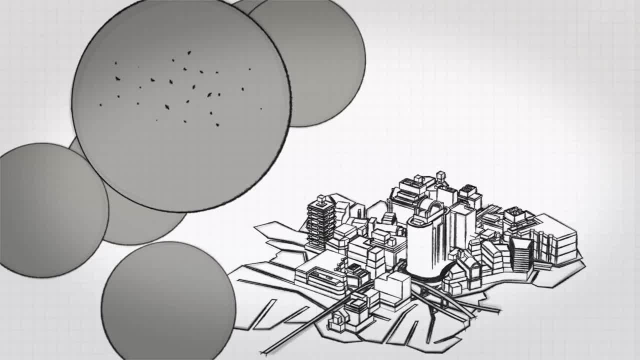 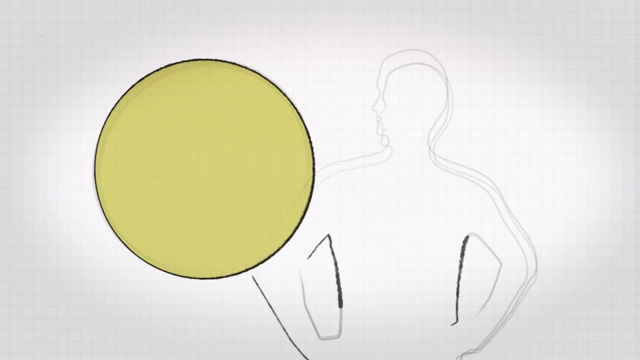 Ammonia in the atmosphere is converted into aerosols, which can travel deeply into lung tissue and cause damage. The formation of aerosols is compounded by urban emissions such as air pollution from industry and vehicular traffic. The smell of ammonia gas is extremely unpleasant. 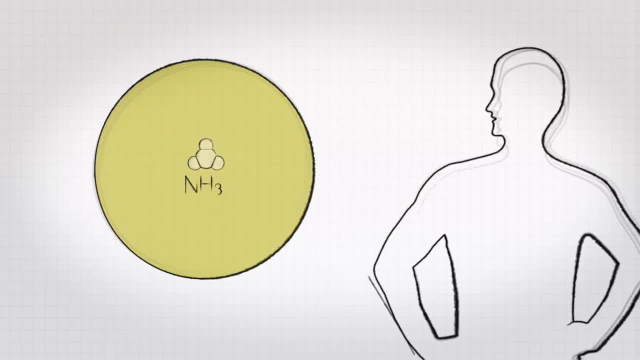 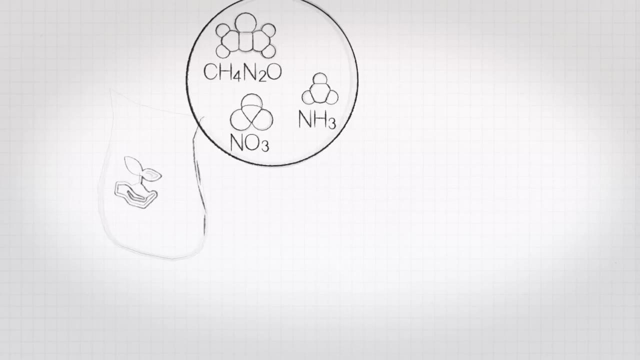 However, this smell helps to keep us from getting poisoned by the toxic gas. Nevertheless, chronic inhalation of small concentrations can attack mucousy, eyes and the lungs and lead to respiratory illnesses. To sum up, reactive nitrogen is valuable and important for plants and humans. 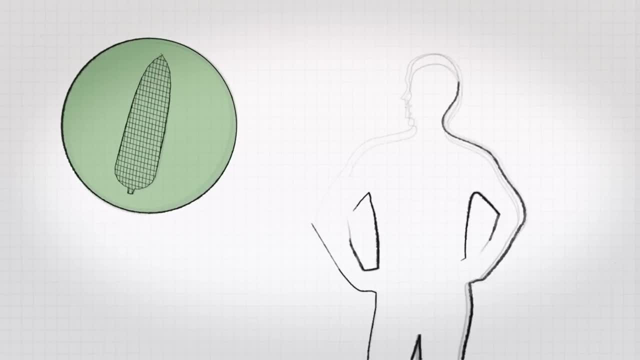 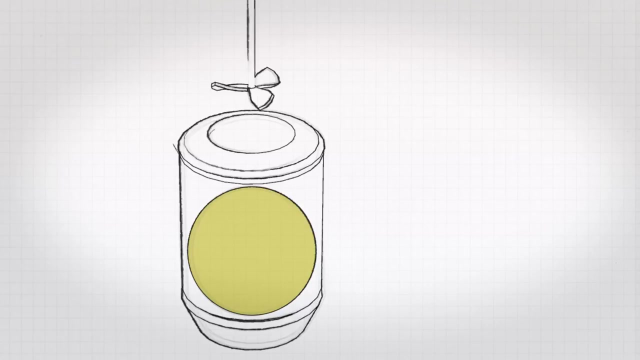 That's the reason why so much is produced in chemicals. Chemicals are used in chemical factories for synthetic fertilizer. Yet if it is excreted and released in abundance into the environment, it becomes a health and environmental problem. When urine is properly stabilized, it maintains its valuable nutrients, limiting the hazardous release of nitrogen into the environment. 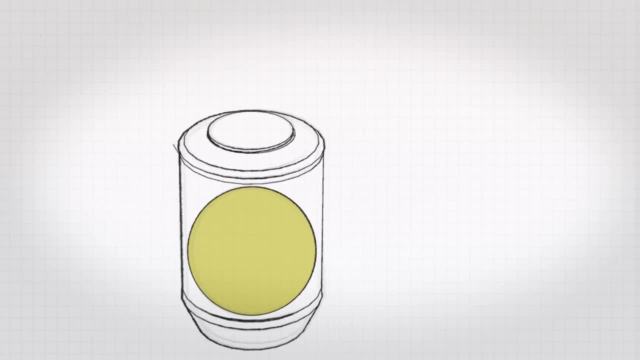 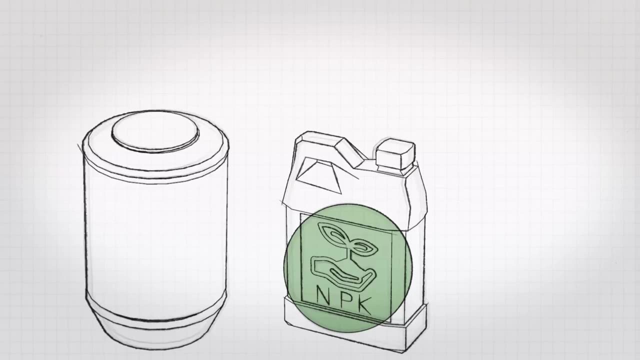 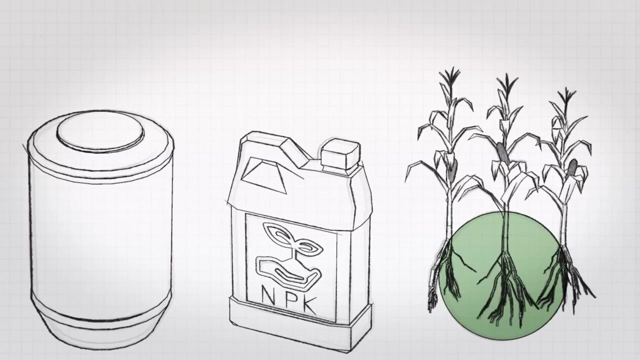 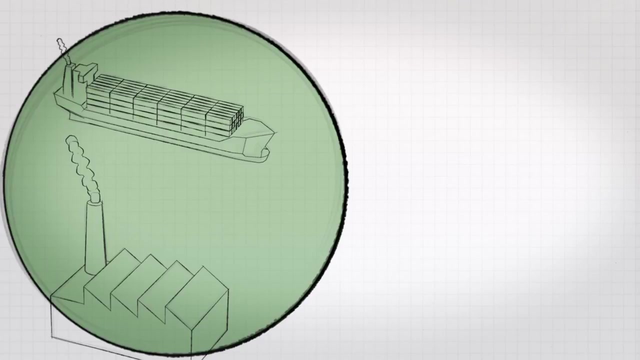 As nitrogen from stabilized urine does not degassify, producing fertilizer from it is not harmful to humans or the environment, And it also does not have malodor. If reasonably applied, the nitrogen can be brought back to sustain human nutrition By closing the nutrient loop. energy-intensive fertilizer production and transport can be reduced. 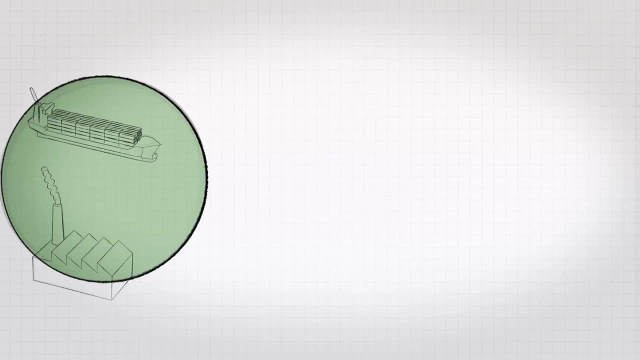 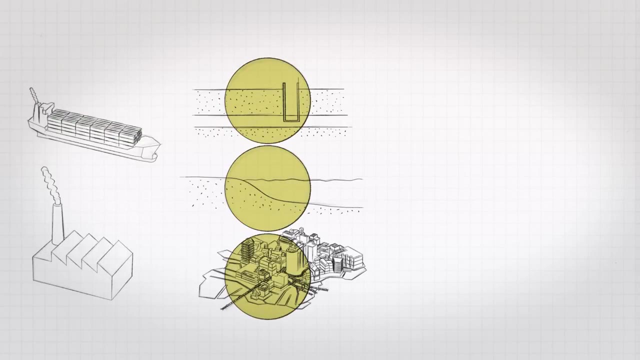 If the production of industrial nitrogen is decreased by recovering nutrients from urine, the discharge of nitrogen into groundwater, open water and the atmosphere is also reduced, And this decreases the potential of future environmental and human health hazards caused by the over-accumulation of nitrogen in the environment.